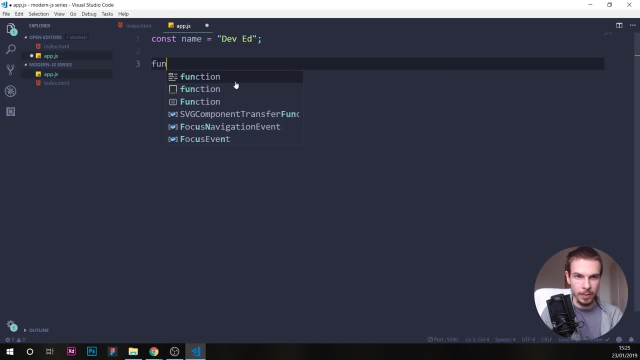 the way we create a function is we're going to write function like so, And again we can give it a name like: let's say, this function is going to take our name here and it's going to put everything in uppercase. All right, So we're gonna name this upper case like so And it's a good convention. 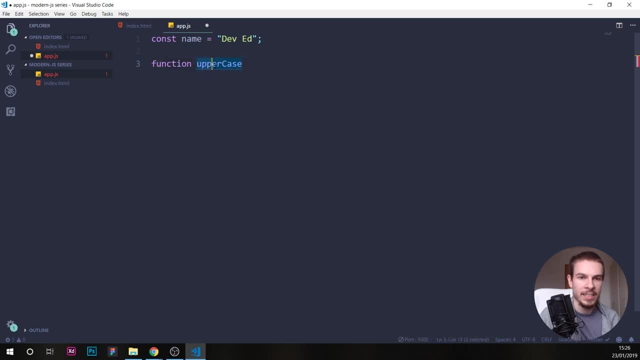 also to use lowercase here and then uppercase here. So let's say, you want to have a variable called gallery images, cons, Gallery images, like so. So this is how we're going to write it, Just because it's going to make. 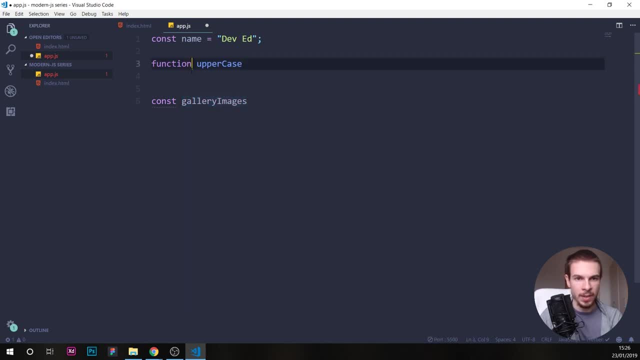 everything more clear. it's going to make everything more visible on what's going on, And it's just basically a convention that people use. So, rather than doing it lowercase like this and then everything just goes together like this, it's going to look ugly and it's going to be hard to to. 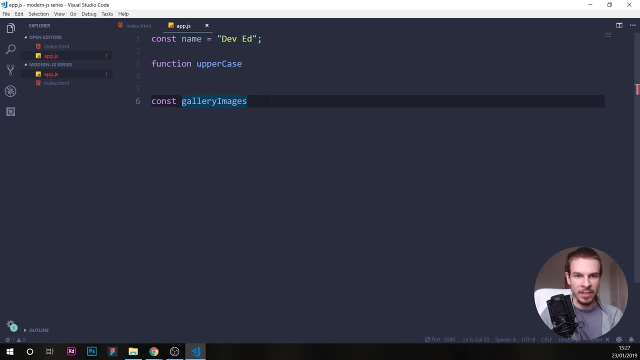 read it And like this it's: everything is just going to be more visible. So, anyways, this is why we wrote it like this, And what we're going to do here is we're going to open up some parentheses like so and then some brackets like so. All right, I'm going to go over what all of these 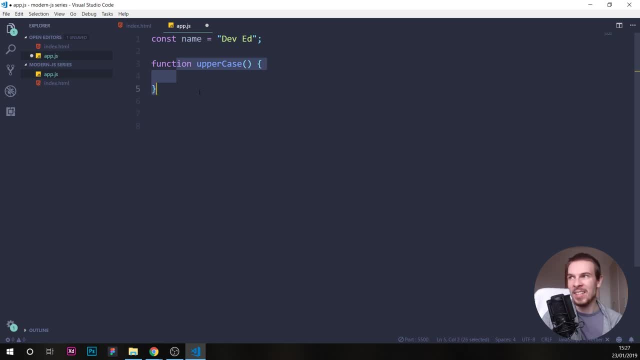 do. But what we did here is we created a function And in here we can give a set of instructions of what we wanted to do. Now let's for now remain this to logger. And here let's say we're going to console log party time, party time, like so All. 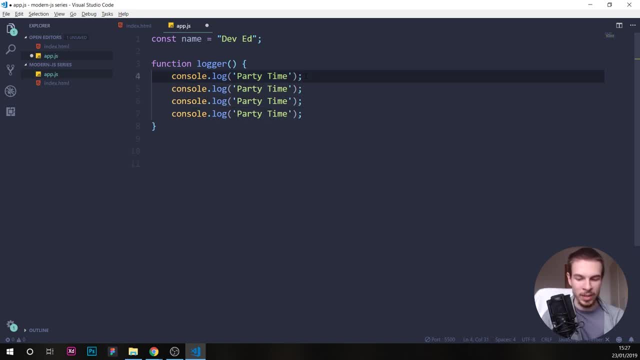 right multiple times. And the way I did that is I just hold Shift and Alt and press down on the down arrow And it's just going to multiply. it's going to create a copy of this down here, All right. so this is our function. it's just going to console log party time. party time four times, Good, But 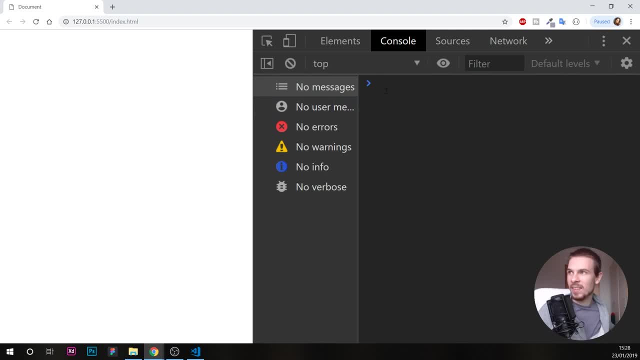 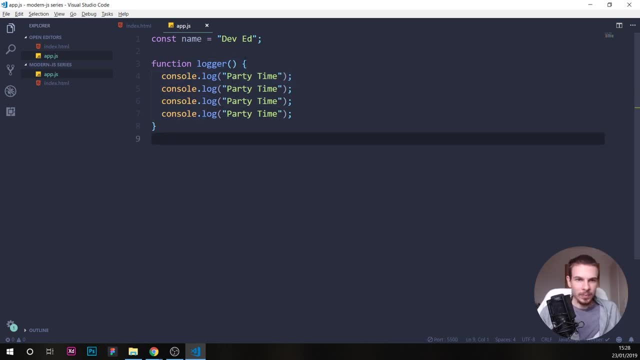 if we look at our code, our console, here, nothing's happening. Why is that? Well, this is not going to execute. So when we run this code, what's going to happen, basically, is JavaScript is going to take a look at this. 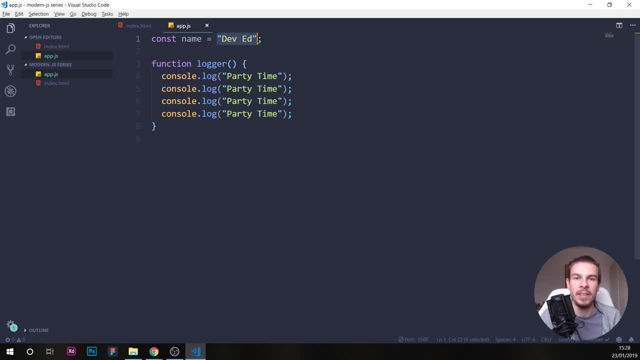 and it's going to say: Oh, okay, so we have a name variable. All right, it has a value of dev ed. Cool, I'm going to save this in memory. Nice, Okay, we have a function here And it has console logs. 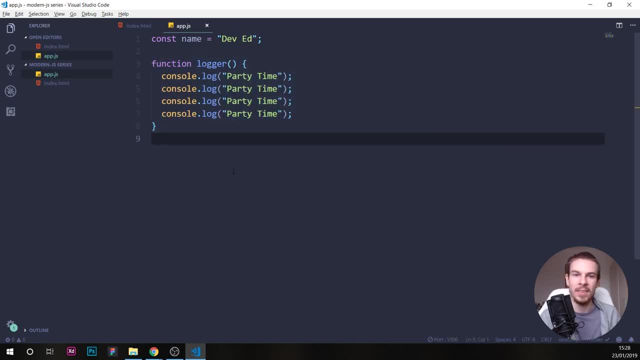 or whatever you want. Cool, I'm going to save this in memory. So whenever we want to run the function, we need to run it. We need to run it. So this is just saving it to memory, All right, it's not actually doing anything right now, So the way we run this code is: 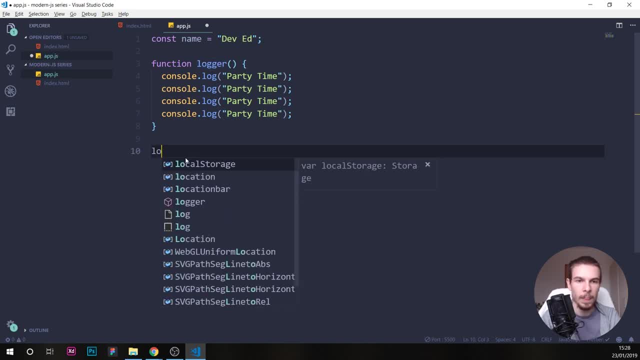 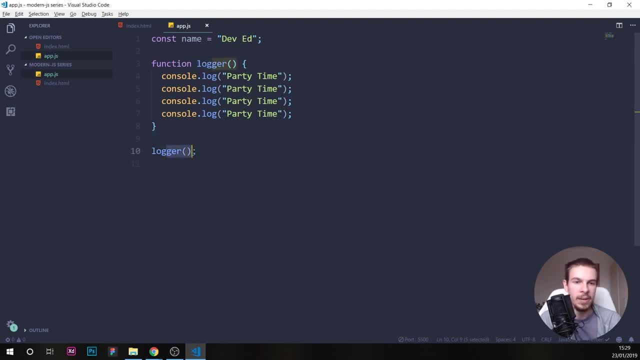 a function invocation. All right, So this is where you want to execute your function. So this is all it does. Cool, But why do we need to add these things here, And why are these brackets here? Well, the thing is that the brackets mean that everything that's available here 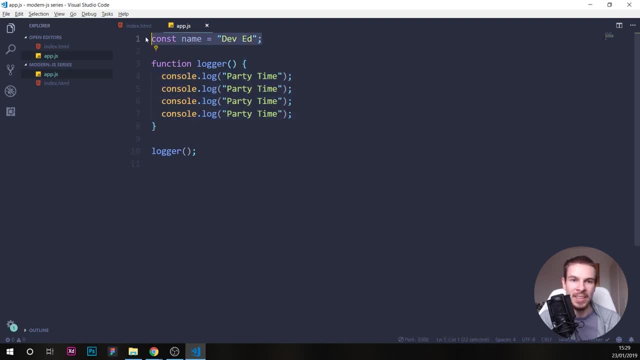 is only available here, And what I mean by that is if we take this const name and add it in here like: so our name down here is not going to be available. So what's going to happen here is we pass the variable in this function So it's only going to be available in here, All right. 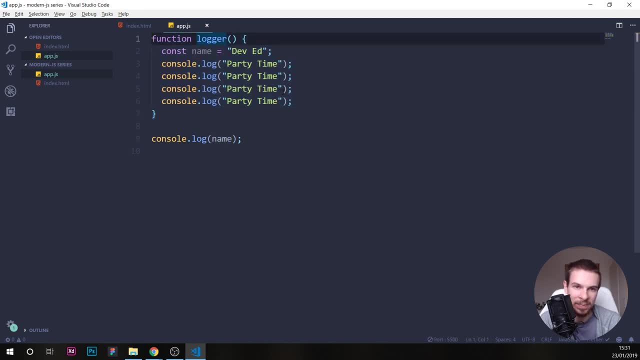 name is not going to be available down here, All right. So whatever variable you add inside the function are not going to be available down here outside of the function, All right. So basically what these are called to quickly go to, this is called the global scope. 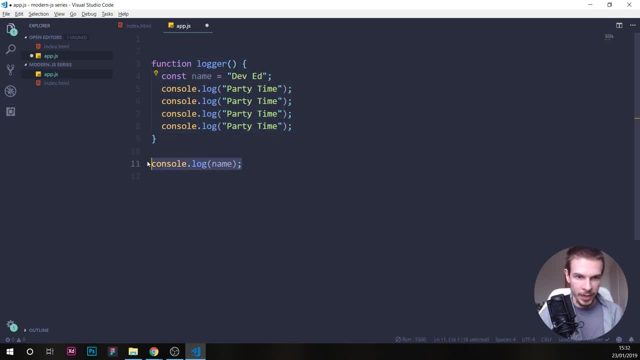 And this called this is called the function scoped. All right So. but however, if you add this to global scope, then in here console log name. so this is going to be available here, So everything from global scope is going to be. 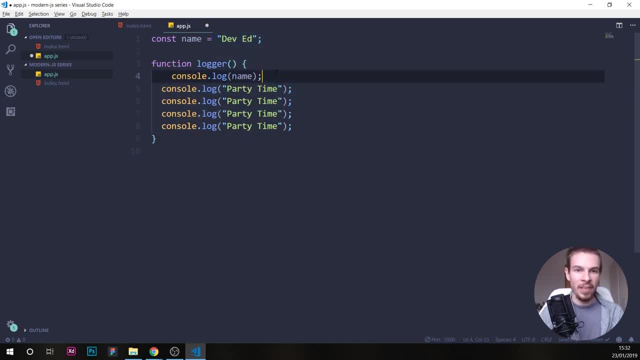 available in our function scope. However, variables declared in our function scope are not going to be available in our global scope. So whatever you have in your function is closed And whatever you have in global is available everywhere. Okay, that's all you need to know. 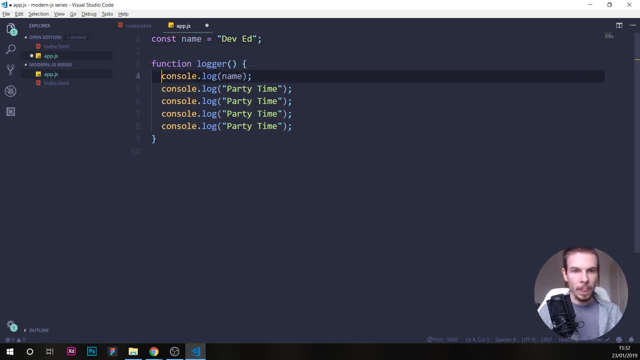 for now. All right, cool, So let's delete this. And why do we need these? Well, now it's the time to change this to to upper. So we're going to do our text to uppercase. Cool, So let's invoke it again here to upper. 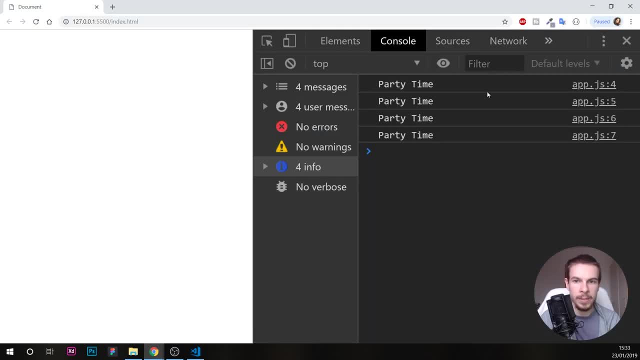 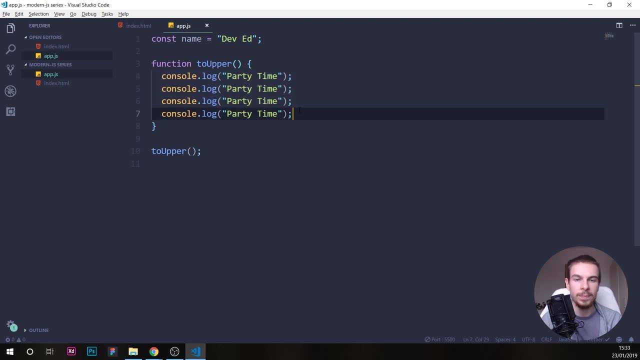 like so close. Let's see if we get party time Good, Or rather than having party time, we want to get this and make it uppercase Cool. So what we can do here is we can add. the reason why we add these parentheses is that we can add a parameter to it. 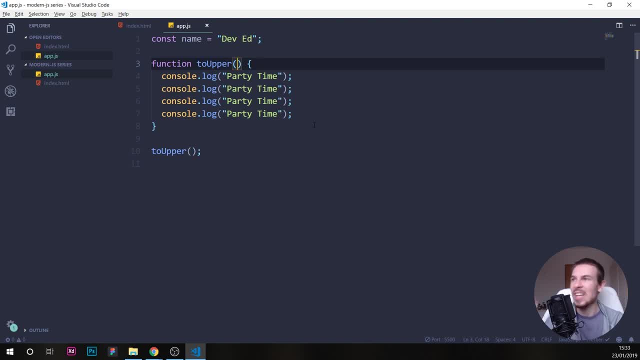 And what the parameter does is basically you can inject a variable or a value inside of it And it's going to run down here. you're going to have access to it down here. So what I mean by that is, let's say, we have 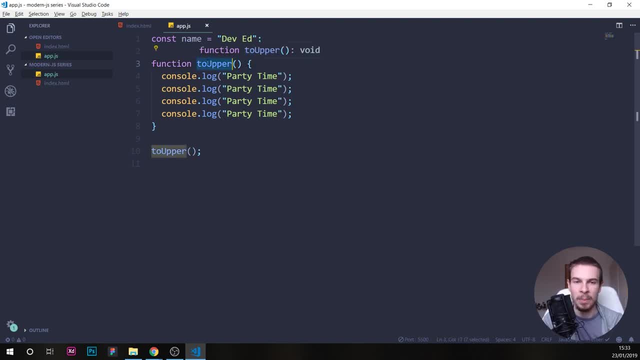 actually let's say: let's say we want to add two numbers together, So two. let's say adder, like so. So here what we can do is we can console log And we're going to say: let's just add two values here, So you can name. 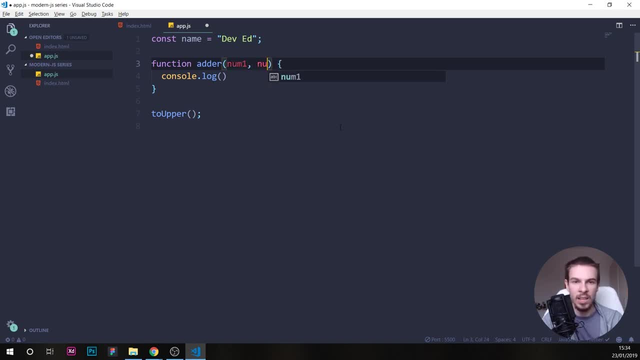 these. whatever you want. You can say number one, number two, with comments. Okay, So here we can console log number one plus number two. All right, Now this doesn't make any sense. What is number one And what is number two, We don't know, And we console log the addition down. 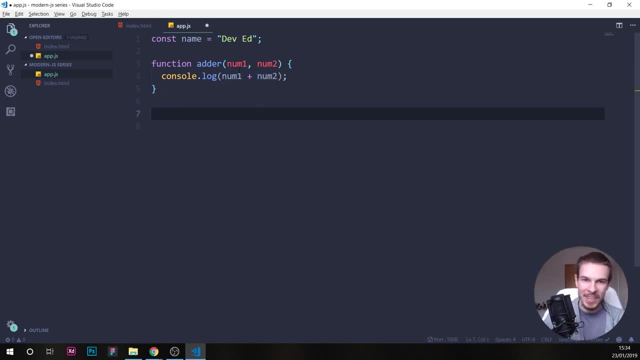 here, Cool. Well, it makes no sense until you invoke the function. So adder here. we can pass in here the two different numbers that we want And that's going to be injected in the parameter here, And then it's going to pass down here and add the numbers together. So if we add five here and five, 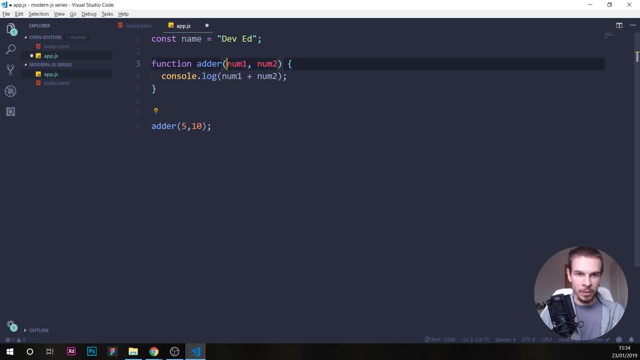 or 10, then the five is going to go in here. So basically it's going to be injected in here, 10 is injected in here and then the console log it's going to add these two numbers together. So if we 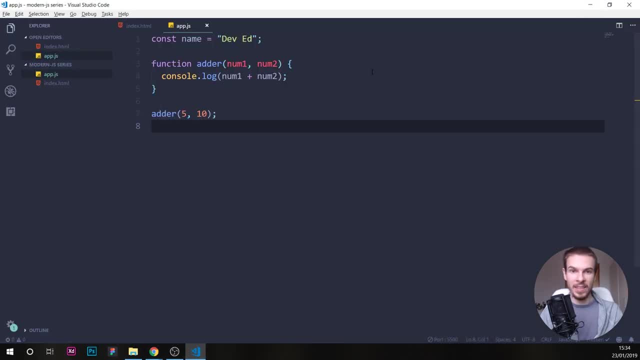 save. we're going to get 15 here, So that's. that's why we use the parentheses, is because we can add different parameters in here. Now, why is this useful? Well, again, if we go back, I'm jumping. 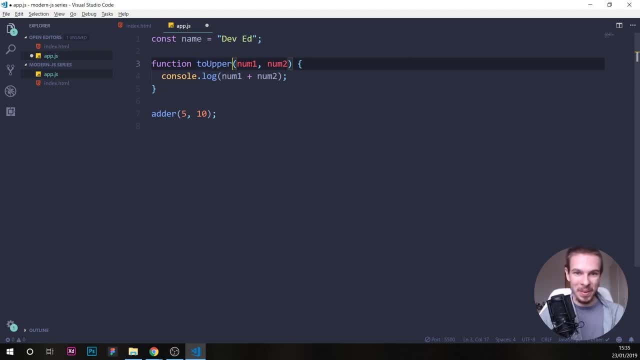 around with this two uppercase 10,000 times. But if we add the two upper, well we know that we are get a text that we want to uppercase. Now we can. we might need different kind of text to be uppercased, So we don't want to just execute it on this And I'm going to show you in one bit. So 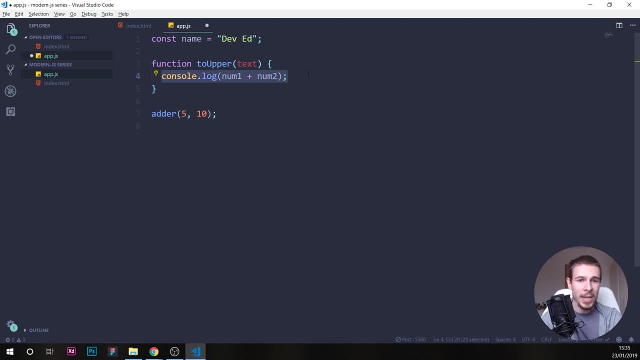 let's just say we have a text in here And what we can do here is we can get the text And if we add dot we can call additional functions that are built into JavaScript. So strings, so text, have different functions built into them. Numbers have different built in functions that we can use. 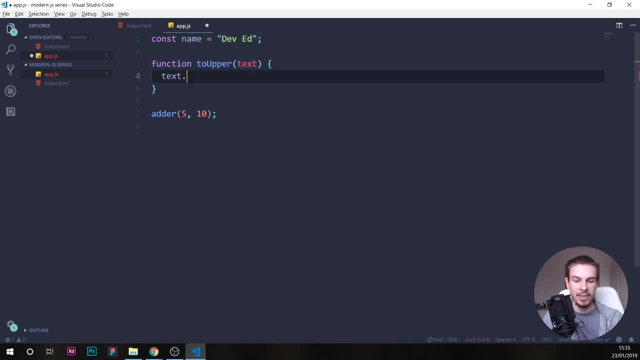 on our code So we can do text dot to upper case like so: And then we do the parameters again. this is something inbuilt in JavaScript That's going to make our text uppercase. So now we can say console log text like so: 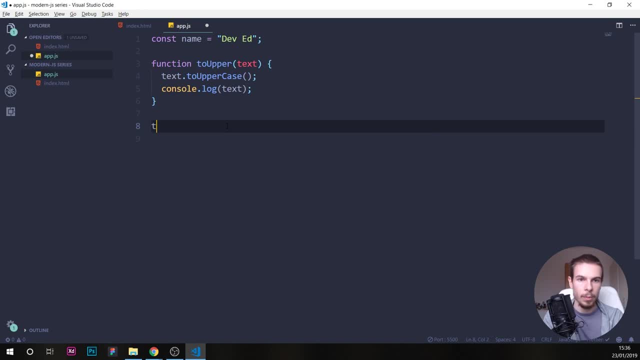 Hit save And down here we can say to upper. And now what we can do is we can inject the name from up here down here. So if we say name and we check, well, actually what we need to do is we can take and create a new variable, Rather than just console logging text, because that 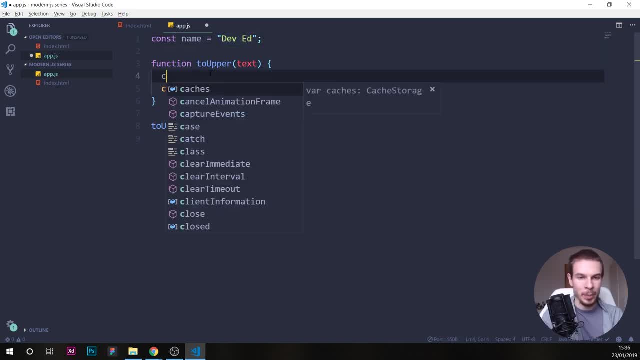 that's the value that's going to be console logged. What we can do is we can create a const called uppercase, Like so. So we create a new variable and this function and we just set it equal to our text that we get from our parameter and then uppercase it, So we can console log uppercase. 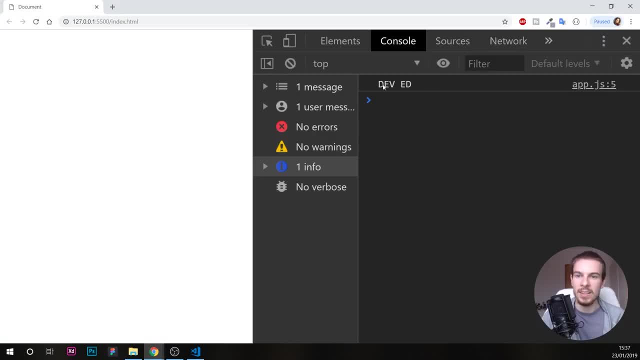 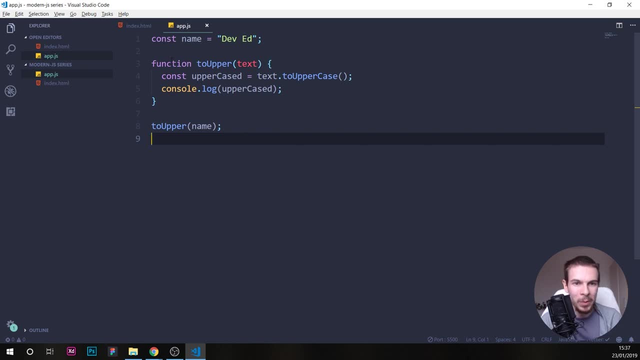 here. So if we hit save, then you're going to see that everything is uppercase like so. So again, to walk through this super fast, we create a function like so. We give it a name. so, just like variables, This is a parameter. Here we create a new variable. 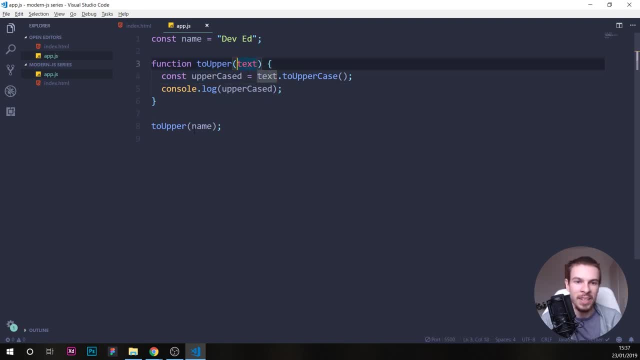 and we just set it equal to our parameter that's going to come in, which is the name. So we're passing the name, this one from up here into here. So this is dev ed here, and then our uppercase is going to be equal to dev ed dot to uppercase. So this is a, again a, a function. 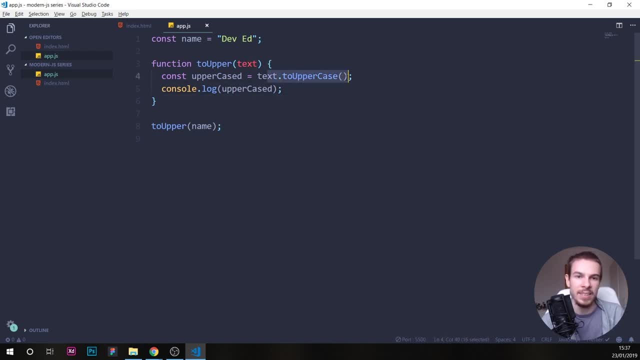 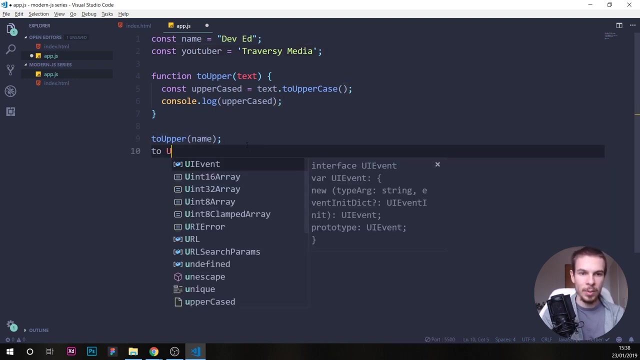 that's already built in for us That we can use on our text, And then we just console log the uppercase. So that's how we can use functions. So the cool thing now is that we can create const. YouTuber is equal to name a YouTuber Traverse Media right. So down here we can just say: to upper YouTuber. 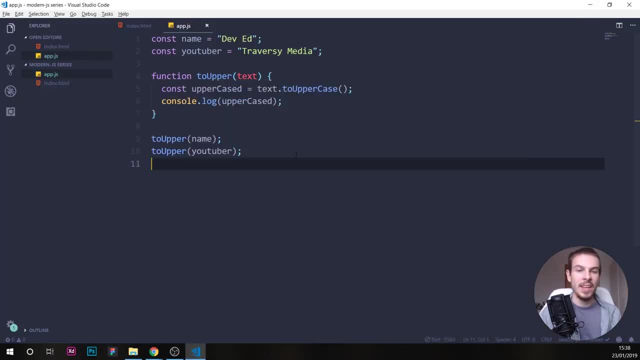 And boom, We have Traverse Media all uppercase. So there we go. That's how that's. that's the basic sub functions that we can use, And later on we're going to cover again different functions that are already built in for us that we can use. Alright, so this is one way we can use a function. 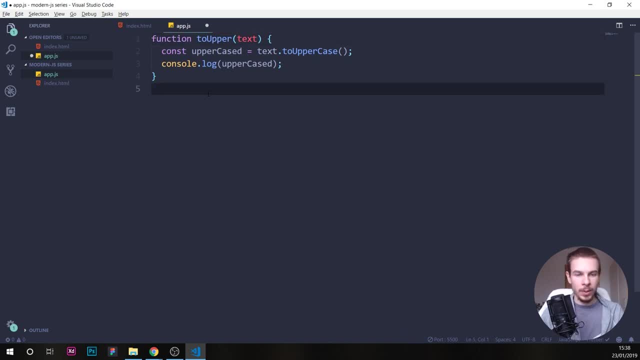 I'm going to delete everything here. Another way we can use one is by doing the way we do variables, which I prefer, actually, rather than this. So then this method. So what we can do is we can do const And we can write, give it a name, So to upper, like: so equal to, and we can set it equal to a function. 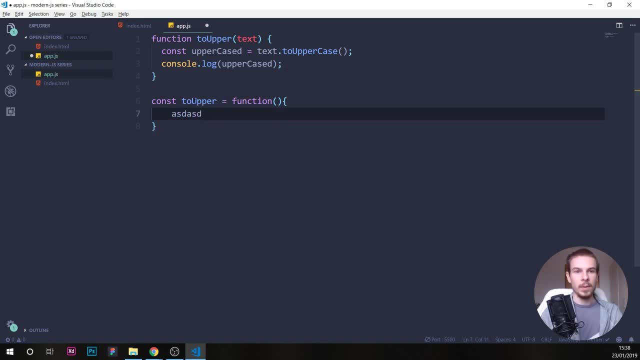 just like normal. Okay, So this is another version you can use And the last version, which is the modern version, we can use. this is, rather than writing this whole function thing, We can make this one shorter, So we don't even need to write function. So what you can replace?